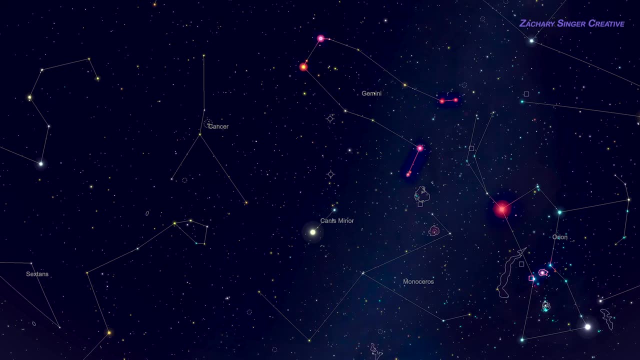 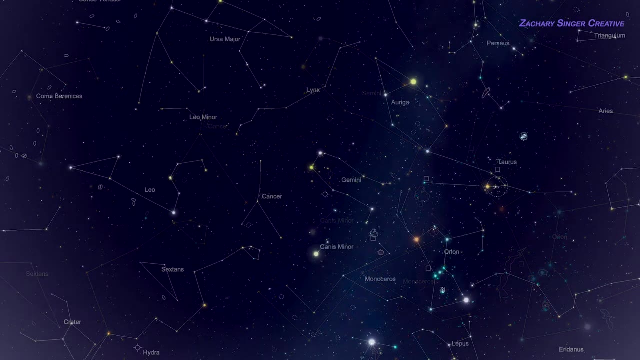 points right at Gemini's feet and Castor and Pollux will be immediately obvious. a short distance beyond them You'll see Gemini very high overhead towards the south around 9pm in mid-February and just a little bit westward in mid-March. The constellation remains visible well into May. though it will have shifted noticeably westward By the time it's left. the constellation will have moved to the north and the constellation will be visible well into May, though it will have shifted noticeably westward By the time of the date. the constellation will have shifted noticeably westward By the time of the date. 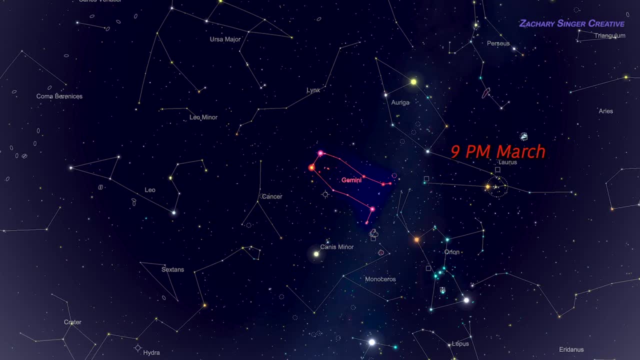 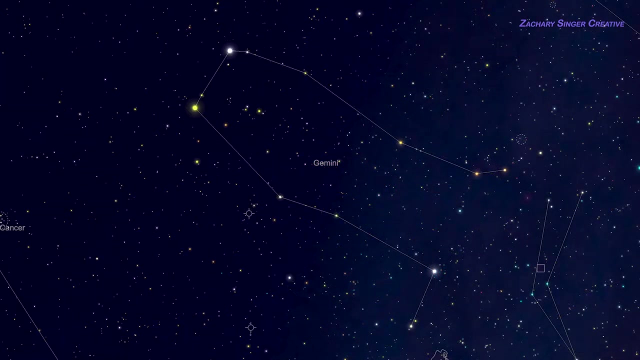 it does, though you'll be so familiar with Castor and Pollux that their new position won't faze you. As we see here, you can also find Gemini at other times of the year if you don't mind observing at later hours or in the early morning. So now that we can find Gemini, 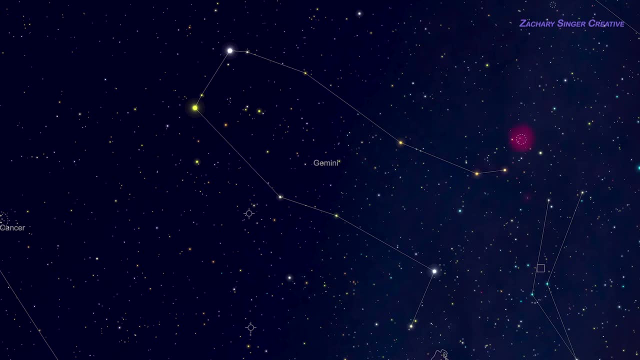 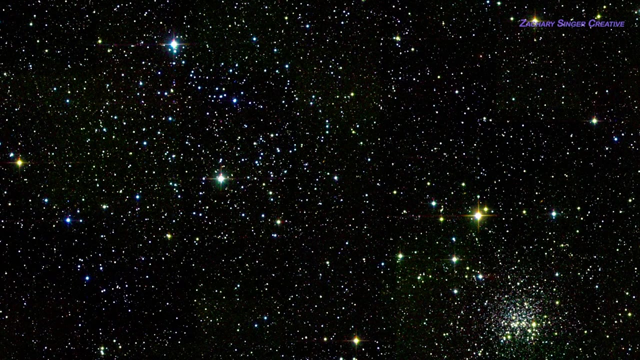 what is there to see here? Well, first, a really great open cluster known as Messier 35, or just M35.. If you have a telescope, even a small four-inch one, M35 makes a lovely target under a dark sky At low power. you may also see a second cluster nearby. This one's called NGC 2158.. 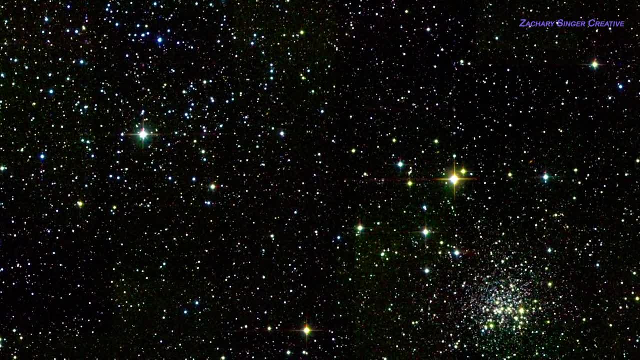 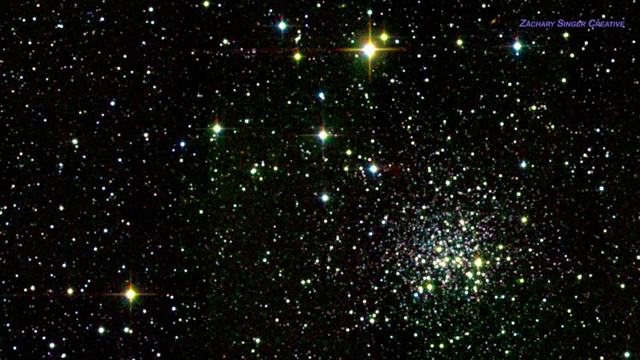 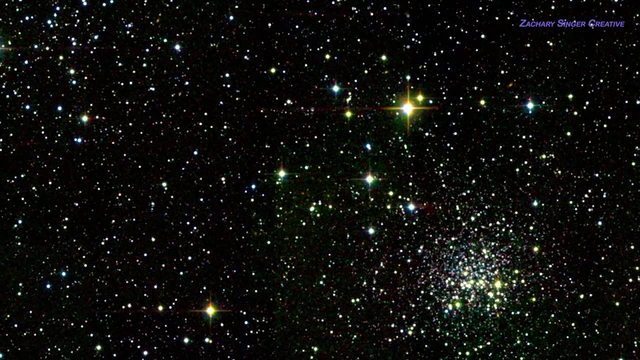 A first-time observer could easily mistake 2158 for a smaller section of M35, but it's actually as big a cluster as M35. It just looks smaller and dimmer because it's at least five times farther away. We don't often get the chance to sense perspective or compare near and far in. 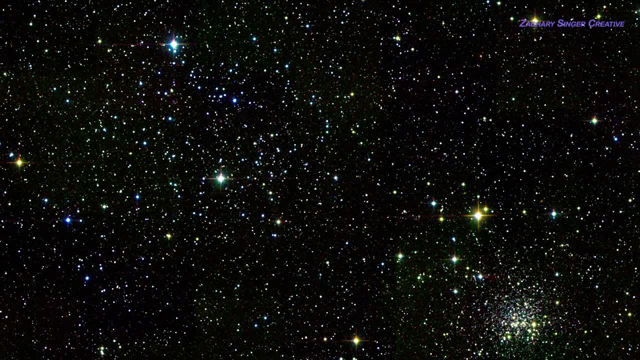 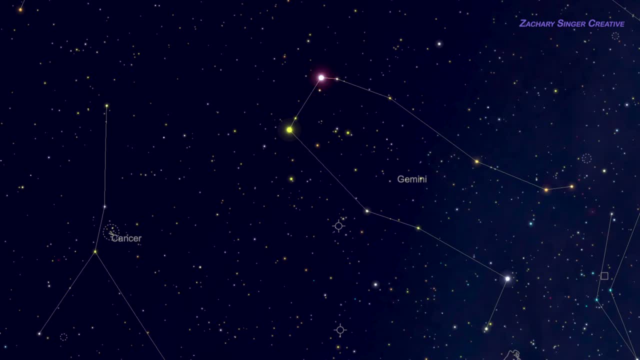 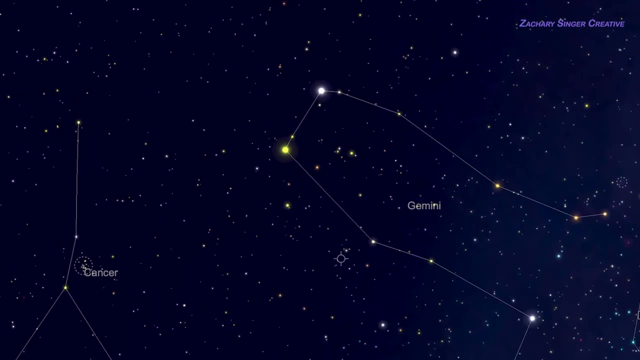 space, but this is one of those times and it's worth a look. Next on our list: Castor, the bright star we've already run across while learning about Gemini. Castor is definitely worth getting familiar with, and not just because it helps us recognize Gemini. For one thing, it's a commonly 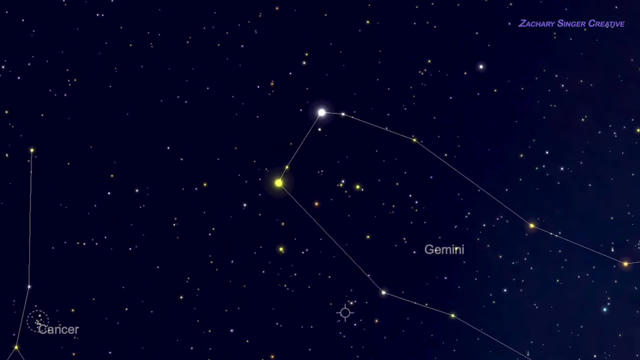 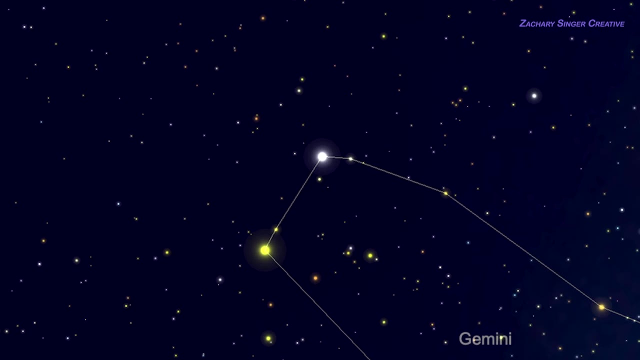 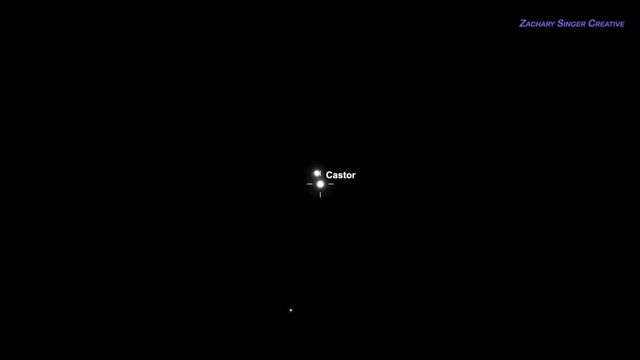 used star for aligning computerized or go-to telescopes. More importantly, it's a star that Castor is a wonderful multiple-star system and quite a sight through even a small telescope. To our eyes, Castor looks like one bright star, but in a telescope a view at 60 power or more.